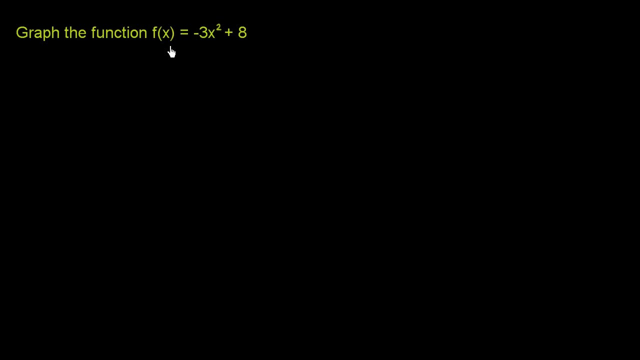 We are asked to graph the function f of x is equal to negative 3x squared plus 8.. So we'll do this by essentially trying out different points for x and seeing what we get for f of x and then graphing it. But the first question I have for you: 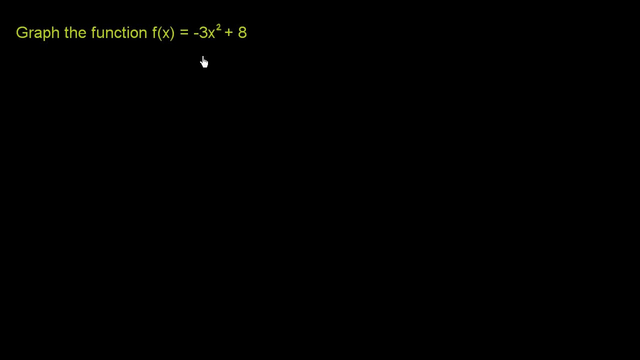 is just looking at this function definition for f of x. what type of graph will this be? Will this be a line? Will this be a parabola? Will this be something else? a circle, something else? maybe something else bizarre or strange? 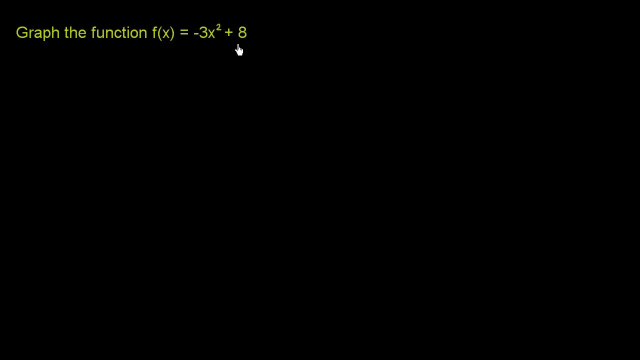 Well, this is pretty clearly going to be a parabola. here The function is defined, It's negative 3x squared, So you have this second degree term here. You don't have any x thirds or x to the fourths or anything else bizarre. 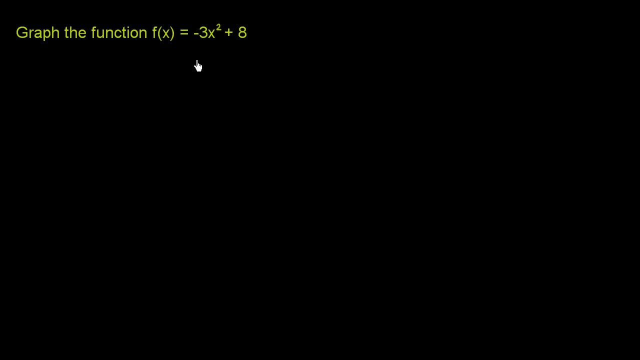 So this is going to be a parabola. Now the other thing that we could think about is whether the parabola is going to open up like that or whether it's going to open down like that. And just looking at this function definition, 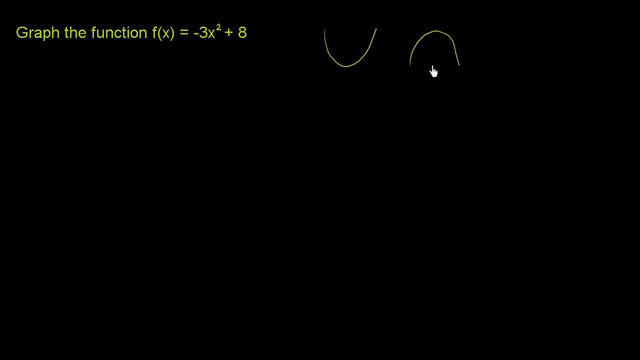 do you have any idea, Do you have any intuition of whether it's going to open up or it's going to open down? Well, if you look at the coefficient on the x squared term, the negative 3,, that tells you that this parabola is going to open down. 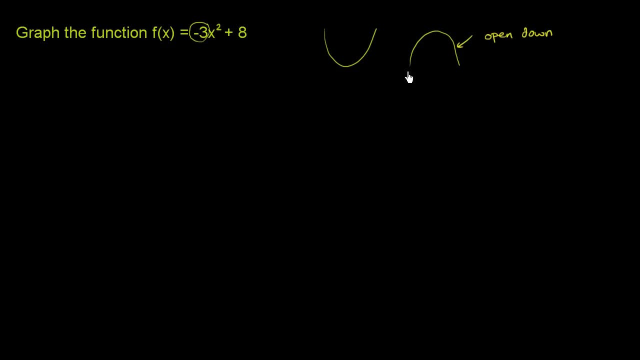 It's going to open down. So with that intuition, now that we know it's going to be a parabola, we know it's going to open down, let's actually try to graph the thing And let me draw some axes here. 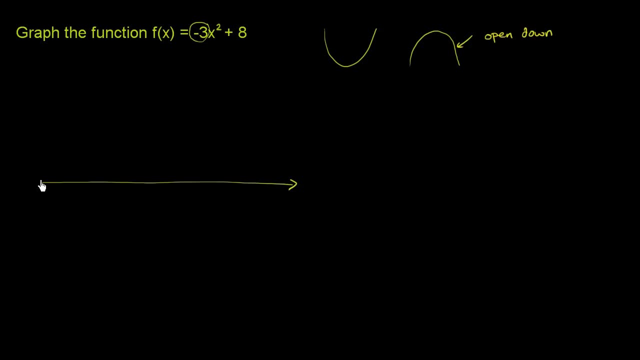 So let's say that this is my x-axis, So that's my x-axis, And then let's make this right over here: This is my y-axis, And let me make a table of values and see what values f of x takes on. 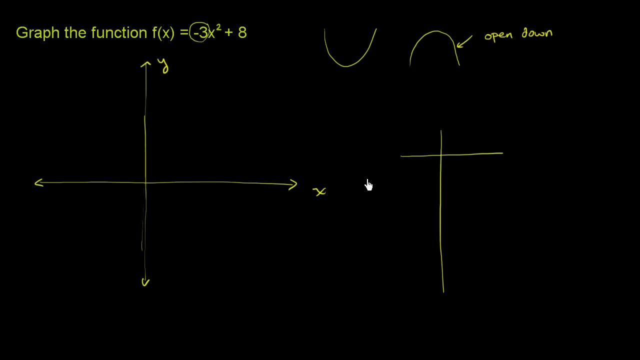 So on one column I'm going to do my values for x, And over on the right I'm going to do my values for f of x, And then we can plot these things. And actually I want to take all of these values before I draw. 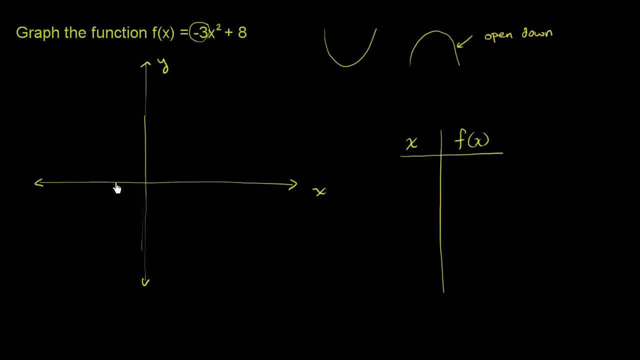 the scale. I want to draw the scale on these axes so I know what might be an appropriate scale. So I'm just going to try a bunch of values. So let's try first what happens when x is equal to negative 2.. So when x is equal to negative 2,, 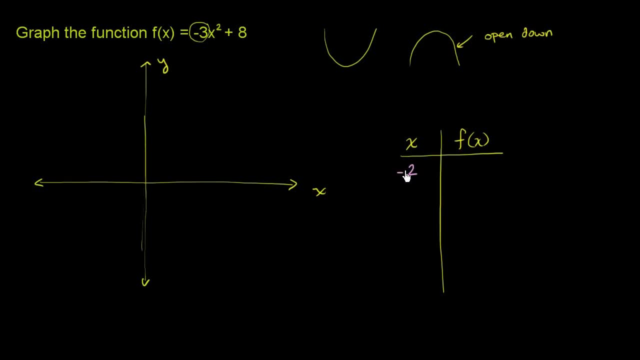 and I'm just picking numbers that will be relatively easy to compute. When x is equal to negative 2, what's f of x? Well, f of x is going to be negative 3, this negative 3, times negative 2, squared. 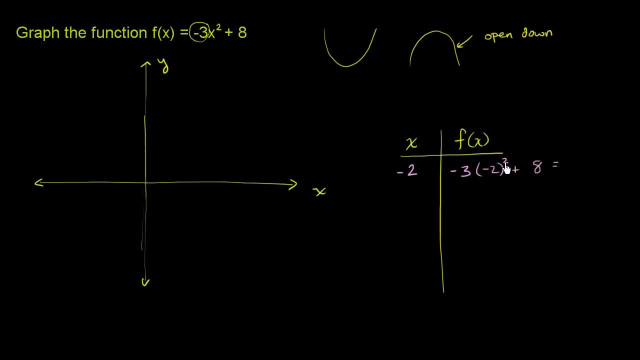 8, which is going to be equal to. let's see: negative 2 squared is 4, positive 4.. Then we multiply that times a negative 3,, which gives us negative 12, plus 8 gives us negative 4.. 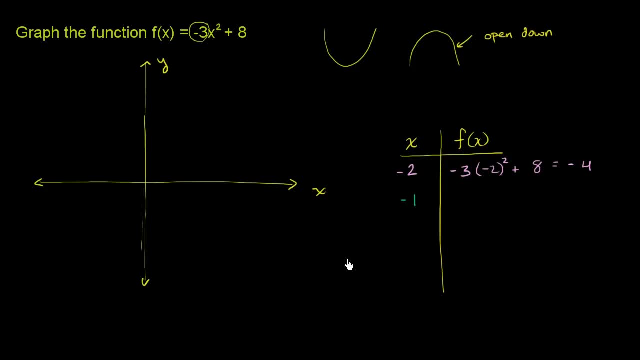 Let's try another point. Let's see what happens when x is equal to negative 1. What do we get for f of x then? Well, f of x is going to be negative 3 times negative, 1 squared plus 8.. 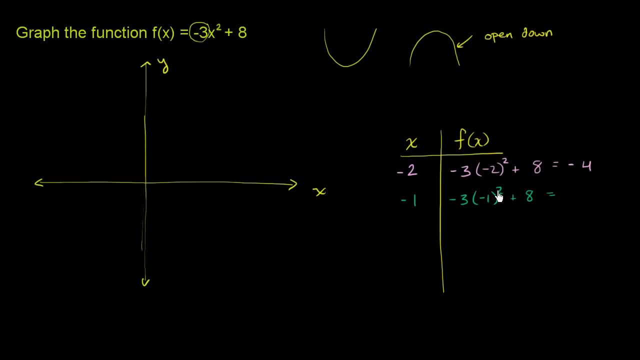 So that's going to be see: negative 1 squared is just 1.. And then that times negative 3 is negative 3.. Negative 3 plus 8 is 5.. Now what does f of x equal when x is equal to 0?? 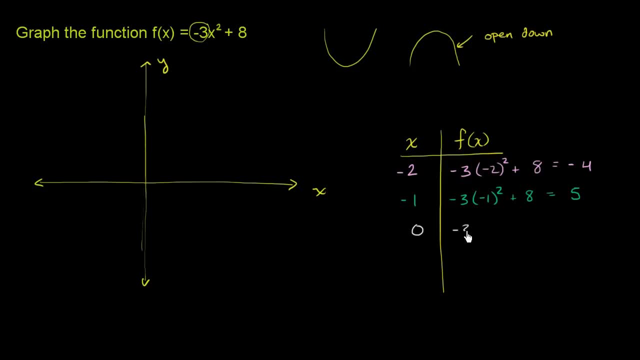 Well, this is pretty easy to compute. When x is equal to 0,, you get negative 3 times 0 squared, which is equal to- and we could write that either way- negative 3 times 0 squared Plus 8.. 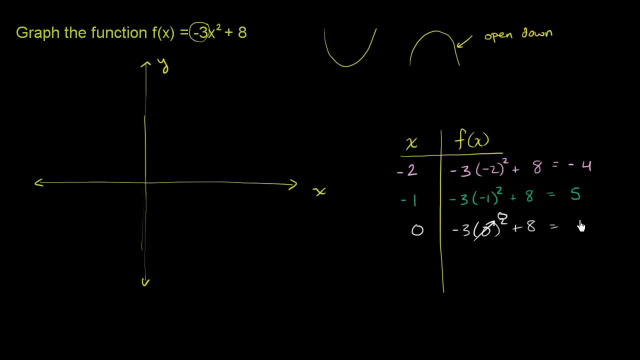 Well, this just simplifies to 0.. And so you're just left with 8.. Now let's see what happens when x is equal to 1.. What do we get for f of x? Well, it's going to be negative 3 times 1 squared plus 8.. 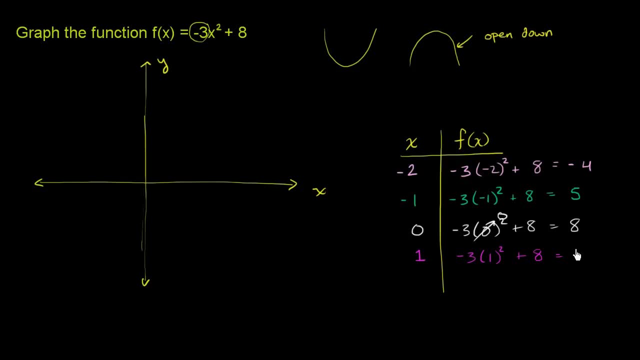 So 1 squared is just 1.. Negative 3 plus 8 is equal to 5.. And then, finally, what do we get when x is equal to Positive 2. What does f of x equal? Or, another way of thinking about it, what is f of 2?? 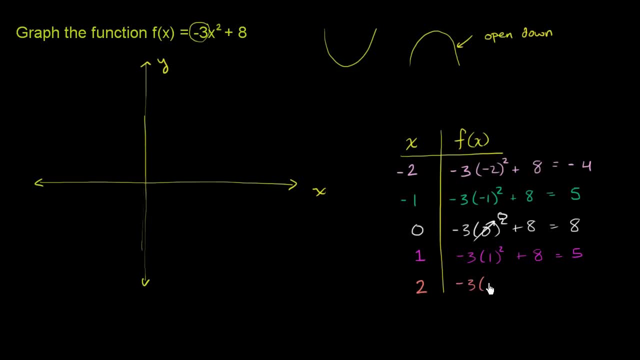 Well, let's think about it. You get negative 3 times 2 squared plus 8.. 2 squared is 4 times negative. 3 is negative 12.. Plus 8 is equal to negative 4.. So let's see if we can plot this. 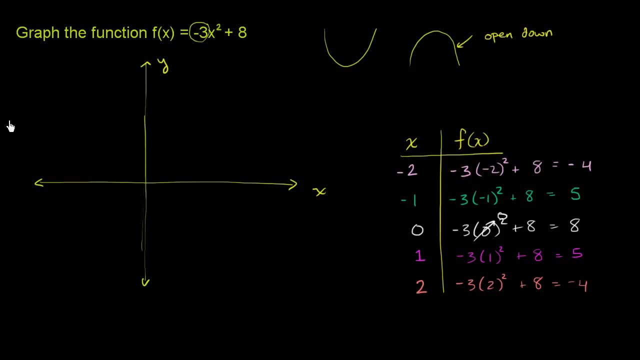 So the x values that I picked go from negative 2 to positive 2.. So let's make this negative 2, negative 1.. This is 0. This is positive 1.. And then that could be positive 2.. And then our f of x values, or we're essentially: 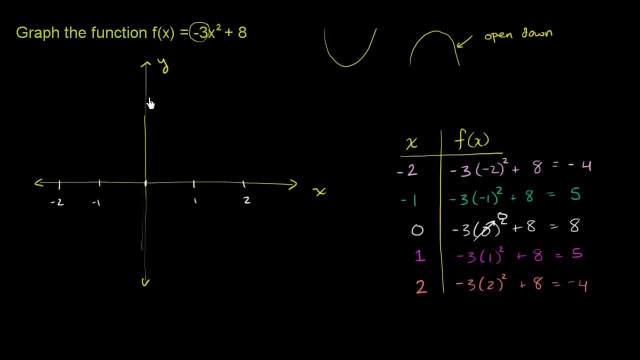 graphing y is equal to f of x. So I can even say this is going to be: the graph of y is equal to f of x Or f of x values. take on things between negative 4 and positive 8.. So let me try to draw that. 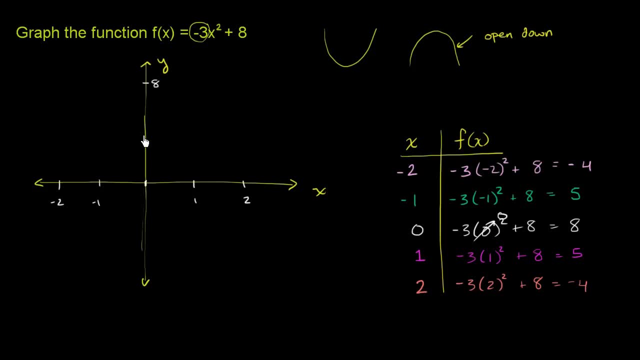 So if this is positive 8, that's positive 8.. That is positive 4.. And then this is positive 2.. This is negative 4.. And if that's positive 4, then this is positive 6.. And then that right, there is 5.. 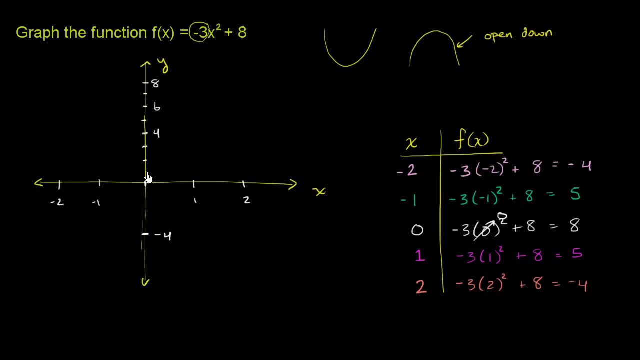 That is 7.. This would be 2.. That would be 3. And then that would be 1.. Now let's graph the points. When x is negative 2, f of x is negative 4. And actually I could say this is the y. 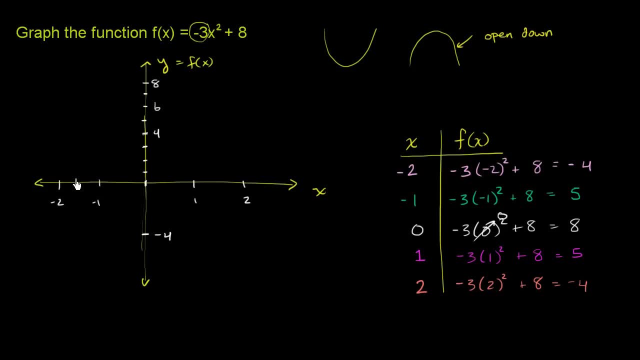 is equal to f of x-axis. I'm going to plot f of x. I'm graphing. This is going to be the graph of y is equal to this function. So let's graph negative 2, negative 4.. So that gets us: when x is negative 2, f of x is negative 4.. 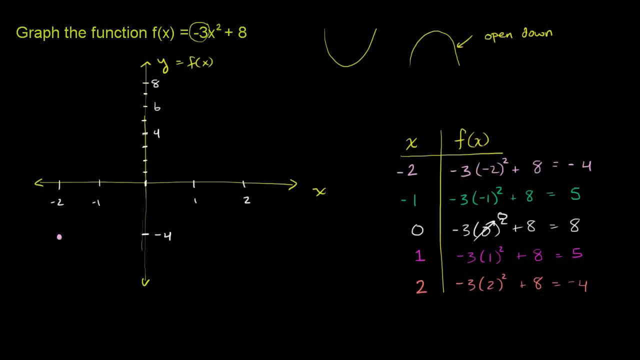 So it's right over there. When x is equal to negative 1, f of x is equal to 5.. f of x is equal to 5.. And we're saying that y is equal to f of x in this context, When x is 0, f of x or y- I could even write over here- 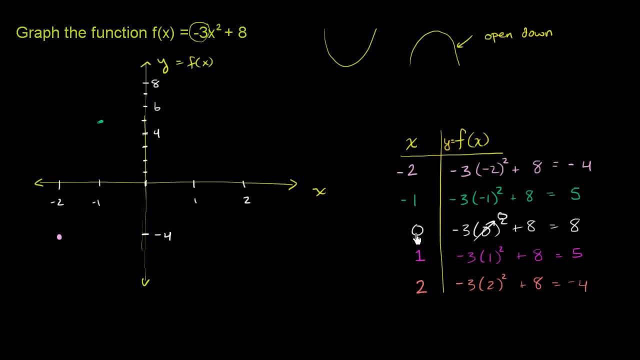 I could say y. y is equal to f of x. When x is equal to 0,, our f of x is 8. x is 0,, f of x is 8.. When x is 1, f of x is 5.. 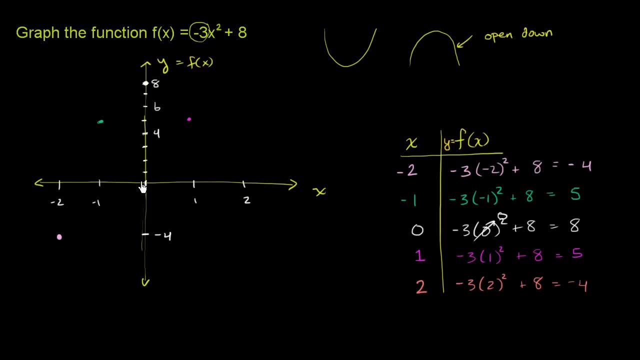 When x is 1, y equals, f of x is 5.. And then, finally, when x is equal to 2, f of x is equal to negative 4.. So 2, negative 4 gets us right there, And now we can connect the dots. 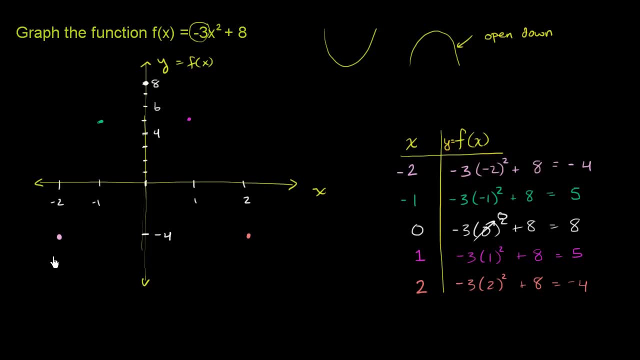 We know this is going to be a parabola And I will do it. I'm going to do it in blue, So my best attempt. I like to draw it as a dotted line, just because it's easier to not mess up.